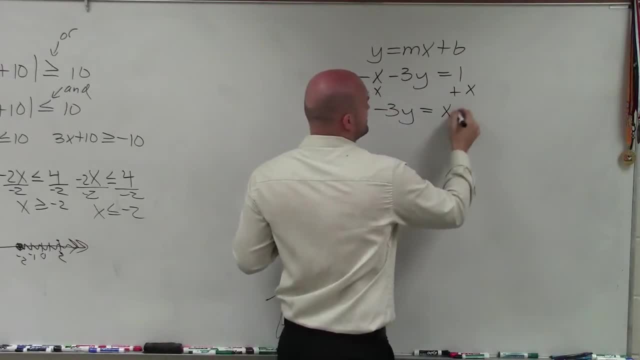 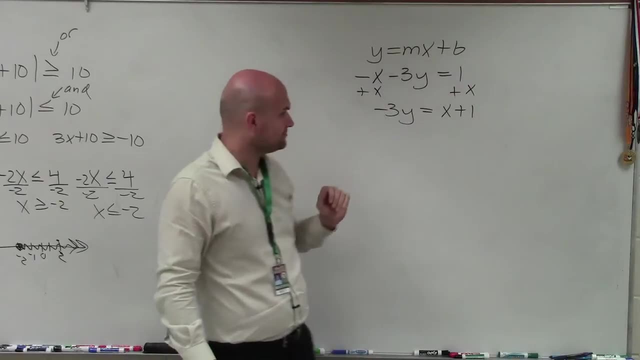 an x. Therefore, I have a negative three. y is equal to x plus one. Instead of writing one plus x, I want to write the x plus one, so my term with my variable is in front of my constant. The next thing is that I want to write the x plus one, So what I'm going to do is I'm 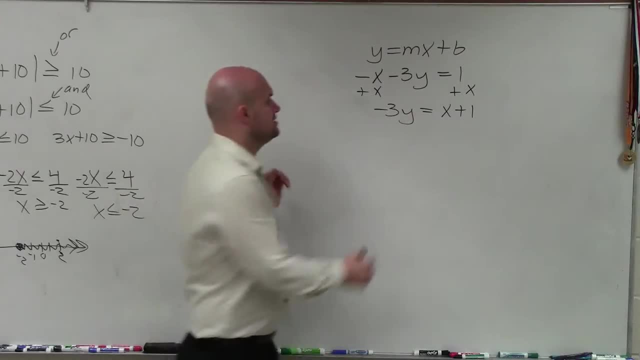 going to divide by negative three on both sides, And it's very important for us to make sure we divide the three into both of these terms and therefore I have: y equals x divided by negative three minus one-third. Now we usually don't write x divided by negative. 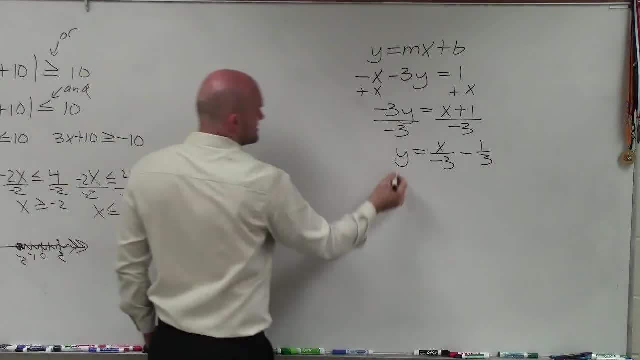 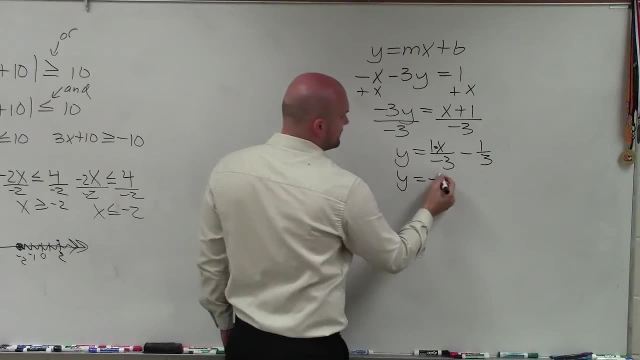 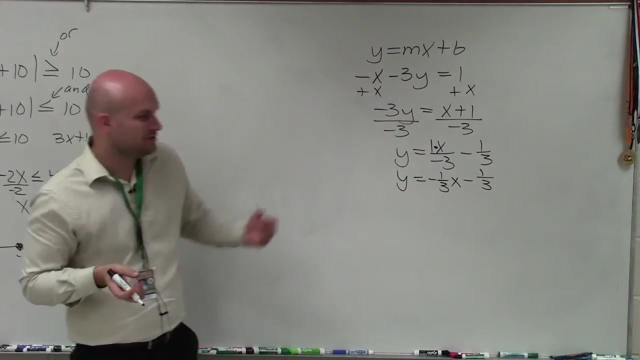 three. What we want to be able to understand is: this can be rewritten: as there's a one times that x And that one times the x, I can rewrite that as a fraction of a negative one-third times x minus one-third. All right, So it's very helpful to understand. so you. 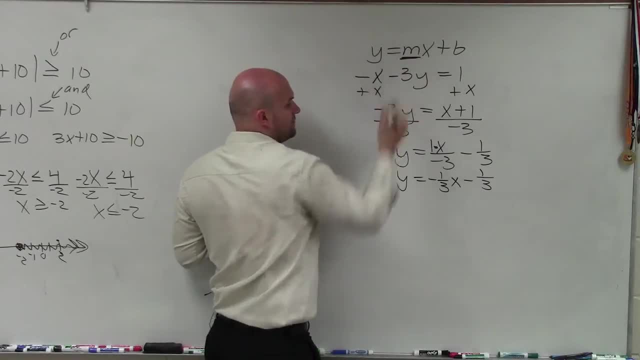 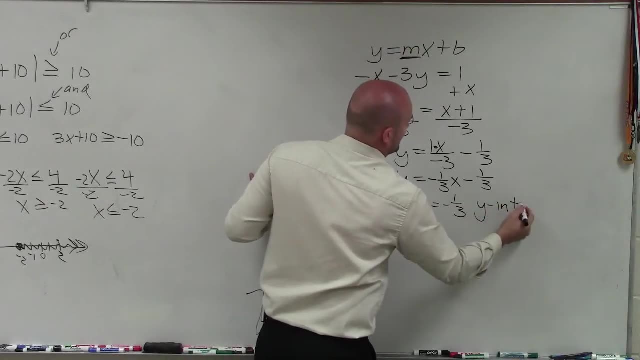 can see where slope, where it's written. as far as m, It's written as the coefficient of your variable, Then I can determine: my slope is equal to a negative one-third and my y intercept is the coordinate point, or y intercept is equal to a negative one-third. 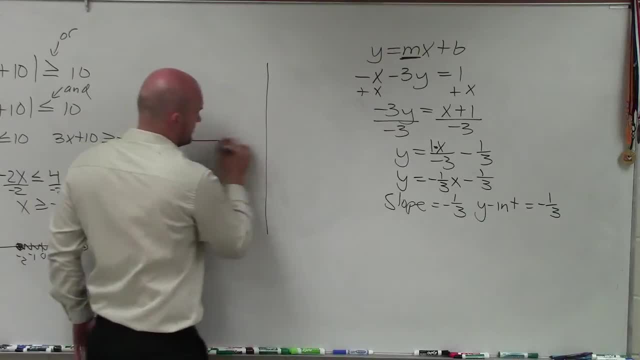 Now remember, the y intercept represents a point. So when I go to graph, I'm going to have: my y is equal to negative one-third and my y intercept is equal to negative one-third. So I'm going to have my y-axis and my x-axis And the first thing I'm going to do is I want 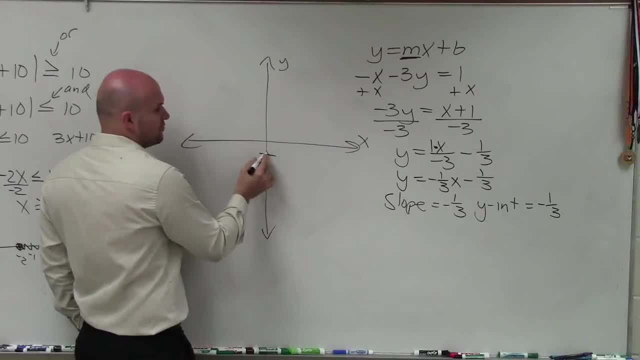 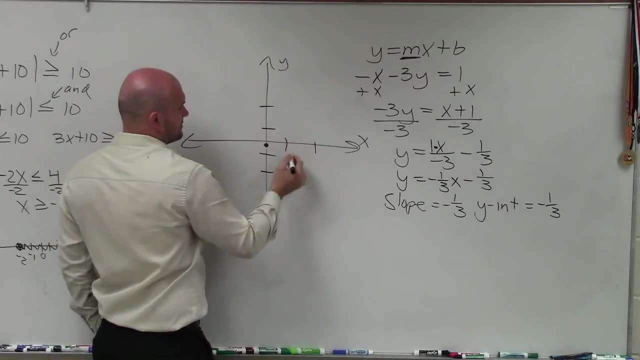 to plot my point at negative one-third. So if I say like here's one negative one-third is going to be right here, Now this can kind of be a little bit confusing. That's a big one, But to graph the points, remember, the slope just tells us what is going to be the 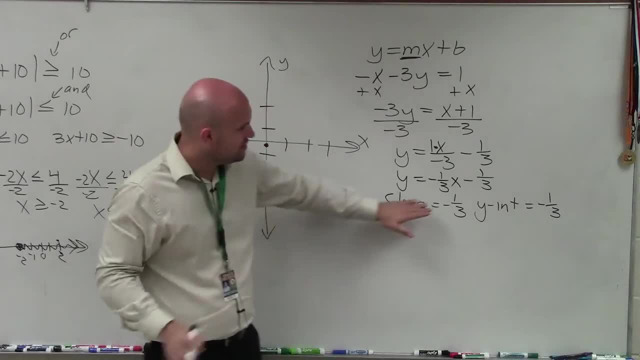 change in your y and your x values between any two points And you have a negative sign. Now this negative sign can be: we can attribute to the numerator And we can attribute to the numerator And we can attribute to the denominator And we can attribute to the numerator. 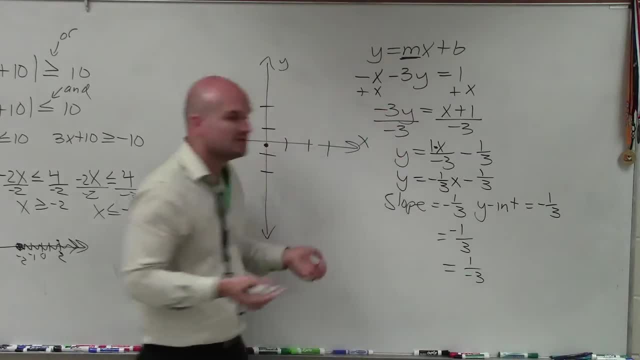 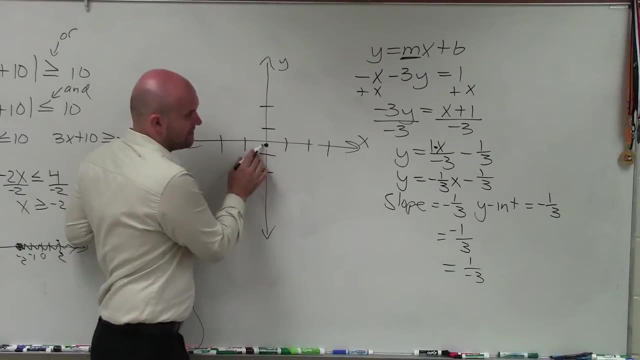 Or we can also attribute to the negative or the denominator, It doesn't really matter. Let's attribute, though, to our numerator for this case. So I have negative one-third If I want to go. if the change in the y values between any two points is negative, one that